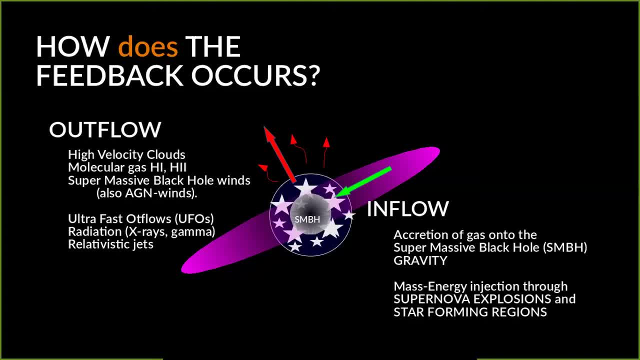 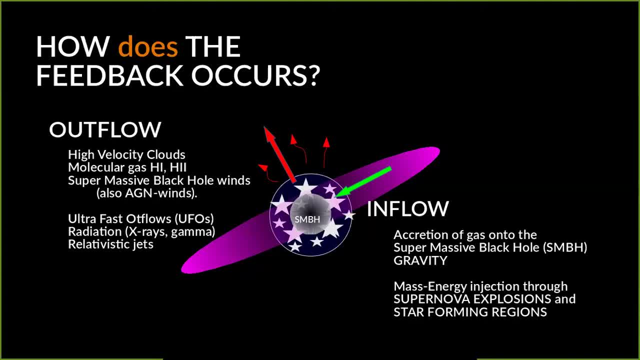 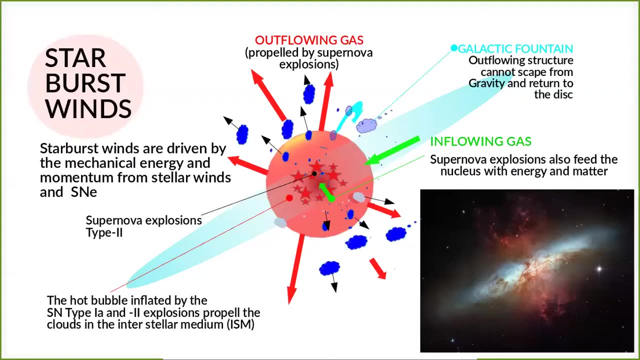 We have inflow of gas filling the supermassive black hole through the accretion And we have outflows being launched from the nuclear region which can be observed as high-velocity clouds, UFOs and molecular outflows. What are the driven mechanisms of these outflows? 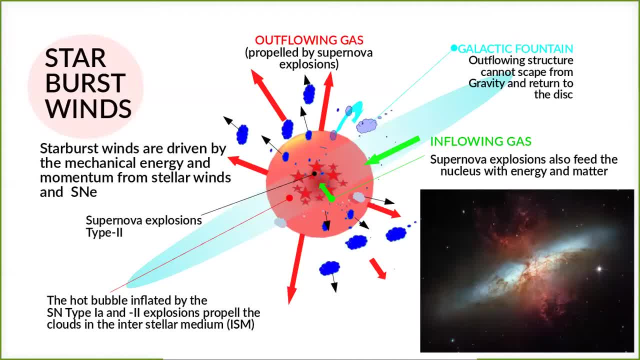 One of them is the starburst wing, which is produced by supernova explosions in regions of high star formation. The massive outflowing gases propelled by these wings are produced by supernova explosions in regions of high star formation, by these winds, and they are seen observationally being accelerated to 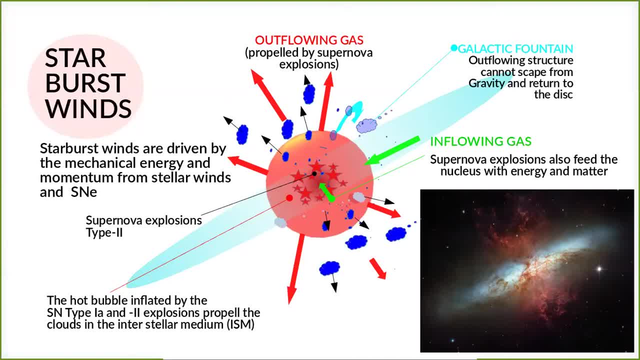 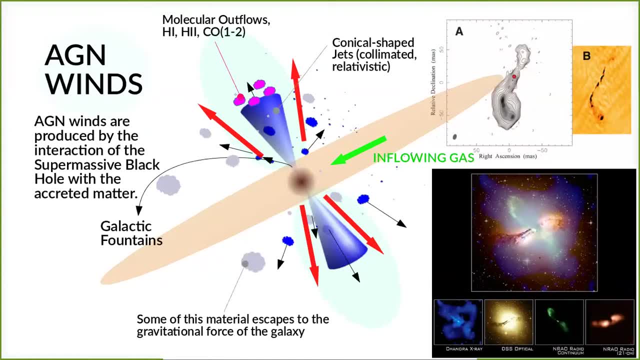 velocities of approximately 500 to 1,000 kilometers per second. Another driven mechanism of urban inaction is the Aegean wind, produced by the interaction of the supermassive black hole with the accreted matter and which are close related to the magnetic fields. There are also objects which show observational 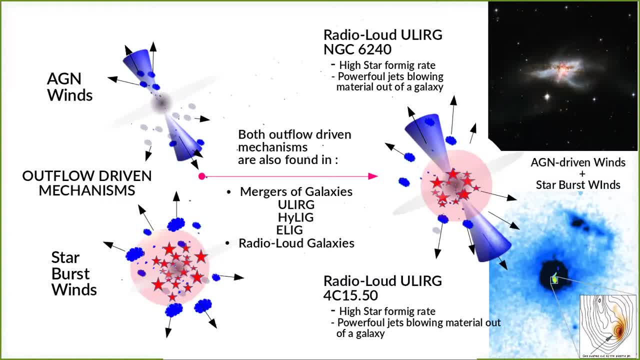 evidence of host both Aegean and starburst winds. Such scenarios are common markers of galaxies, as in the case of the very low ultra-luminous infrared galaxy NGC 6240 on the top. We are very interested in these objects because we want to answer. 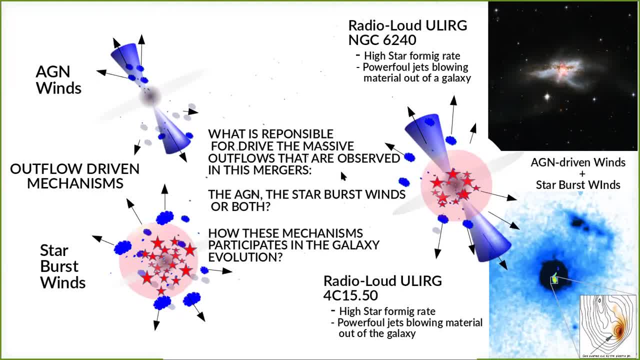 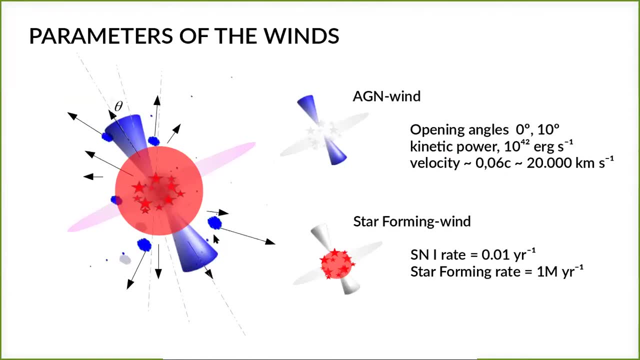 what is the responsible for the massive outflows that are observed in these mergers, when these objects host both Aegean and starburst winds? For this we use the parametric space, the observer parametric space. for the Aegean winds and for the star driven winds We use numerical simulations to 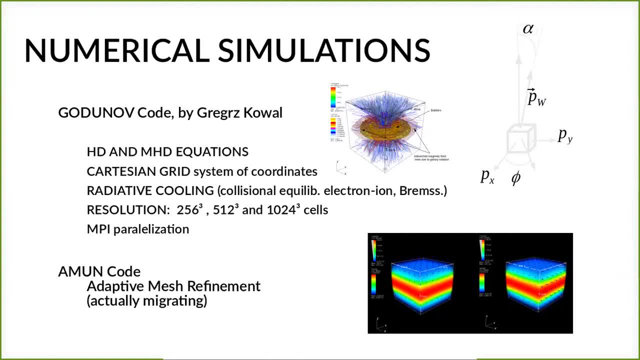 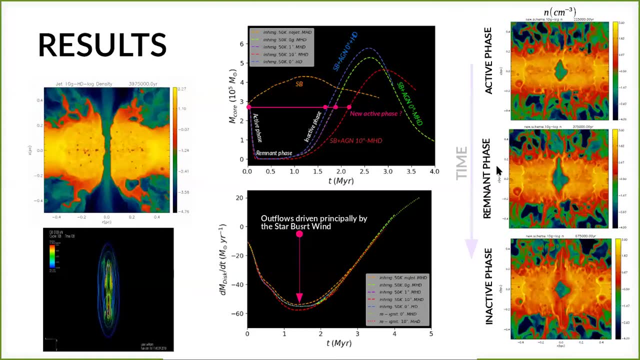 simulate the Aegean wind and the star driven winds. We study these environments using the Grunov code, which resolves HD and MHD equations in a Cartesian grid with radiative cooling and collisional equilibrium. Results One: all the models which host starbursts are Aegean removes the mass. 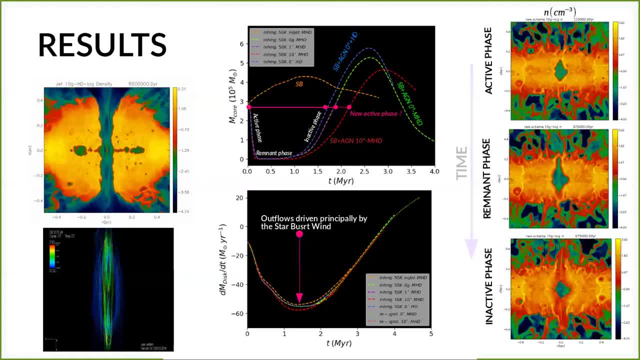 in a nuclear region of 40 parasites in approximately 250,000 years. This contaminates the Aegean wind activity. Two after that, the Aegean wind is inactive, but the remaining Aegean wind still propels the gas to the other regions. In the inactive phase, where the Aegean wind remains, has mixed. 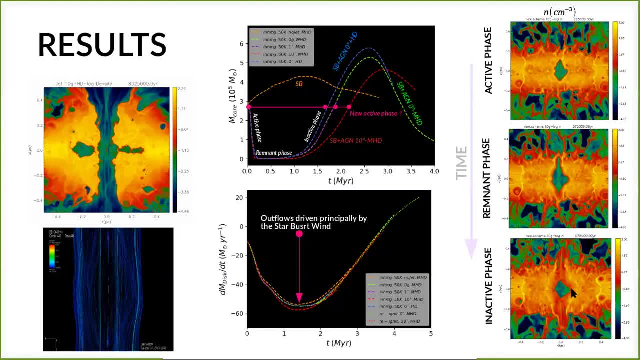 with the interstellar region and the halal region. the stellar activity feeds the central region with gas, inducing a new possible active phase Results. So and so. The mass outflow rate above the disk is not affected neither by the passage of the gene. 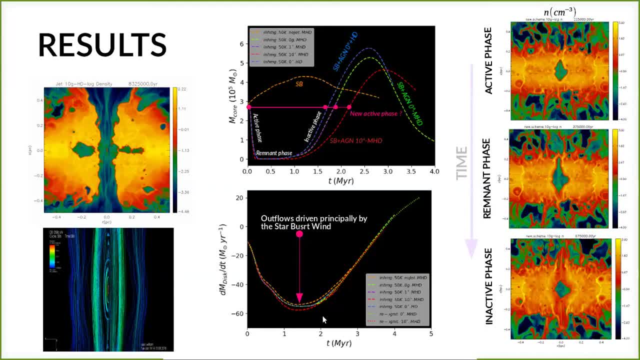 or the presence of the magnetic field. It's only and principally driven by the starburst beam. Thank you. 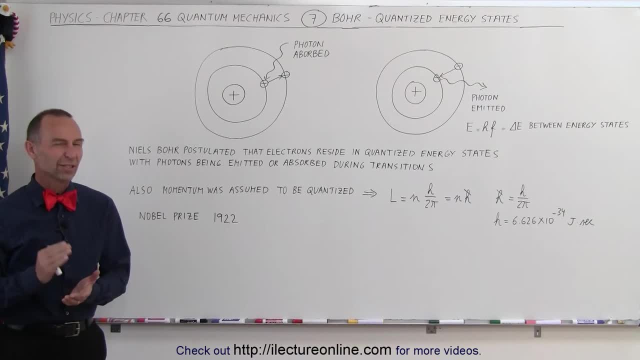 Welcome to Electron Line. It is no secret that in quantum mechanics Niels Bohr was a big contributor to our understanding of the basic structure of atoms, especially when we come to the hydrogen atom, And the result of that was that he postulated that electrons 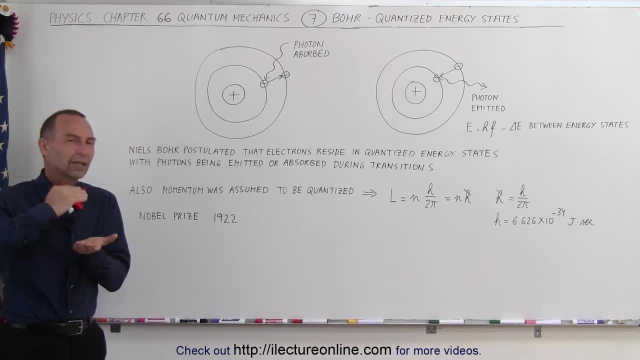 resided in energy levels that were quantized And when electrons jumped from one level to another level, that either a photon was absorbed or emitted, depending upon if the electron was in a higher or lower energy state. Case in point: let's assume a simple hydrogen atom. 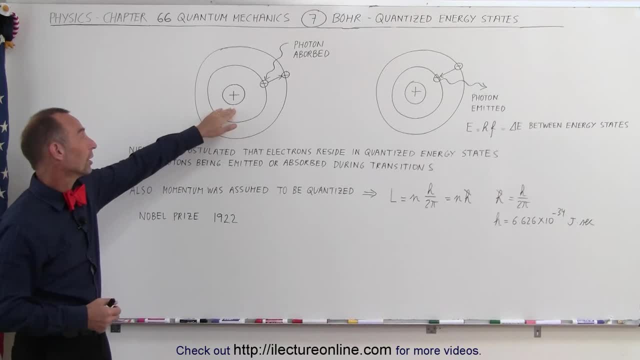 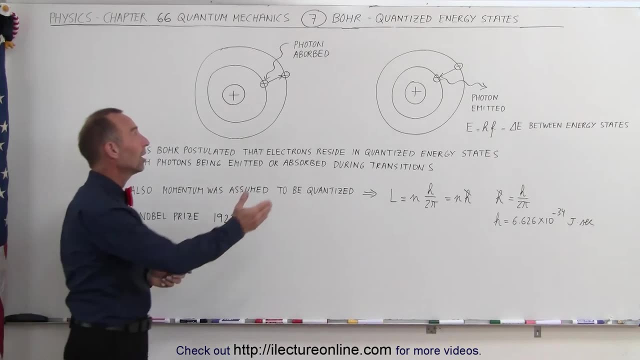 right here. Here's the proton in the middle, which is the nuclear center of the atom, And then we have what he assumed to be energy states in which electrons could exist. And so, for example, if an electron were to go from a lower energy state to a higher energy, 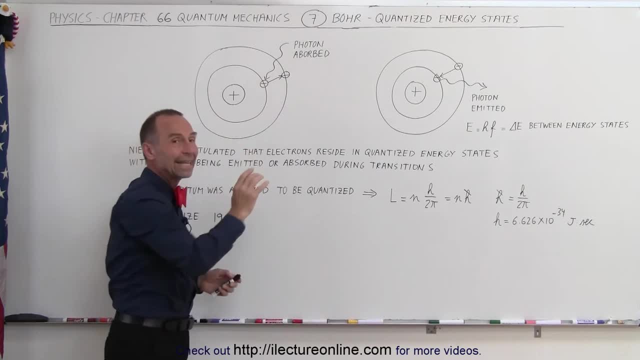 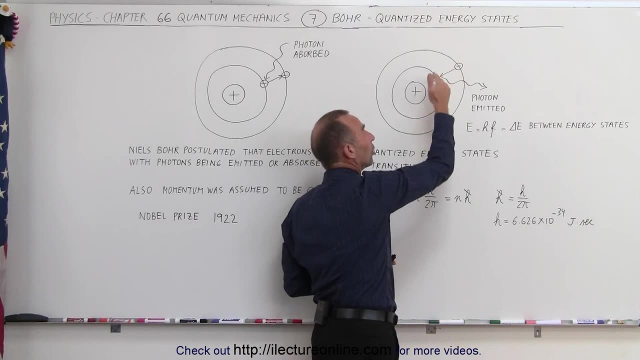 state, it could only do so by absorbing a photon containing that exact difference in energy. Likewise, when an electron would jump from a higher energy state to a lower energy state, to a lower energy state, it would then release the exact energy difference, again in the form of a photon. And remember that they had discovered through Planck and Einstein.